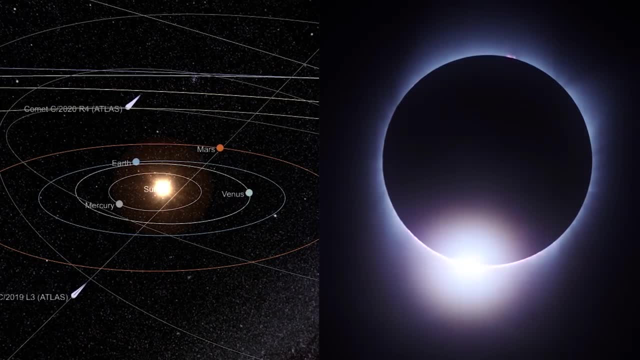 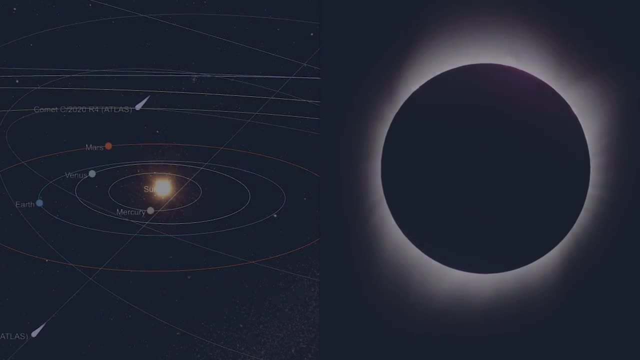 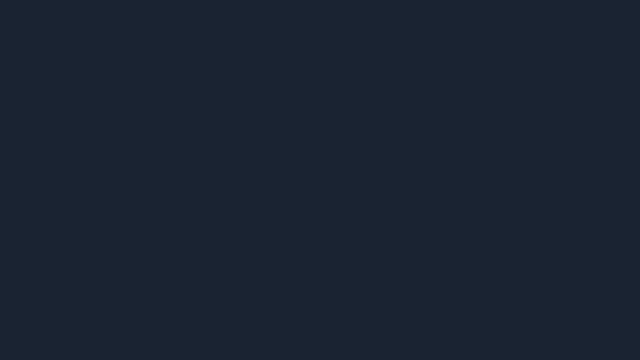 simulations to predict what happens in the real world, or else it may result in a wildly inaccurate, completely different prediction. This is due to the simple fact that these systems are chaotic. The systems that were mentioned earlier are what's known as chaotic deterministic. 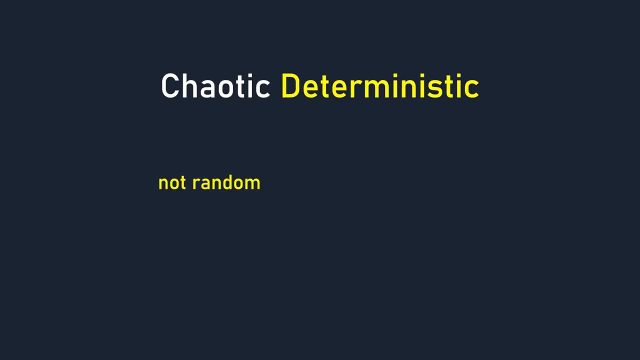 Deterministic means that they are, in fact, not random. Given any initial conditions, there is one and only one way that the system will pan out. However, the fact that they're chaotic means they display aperiodic behavior over time, meaning there's no observable pattern as to how. 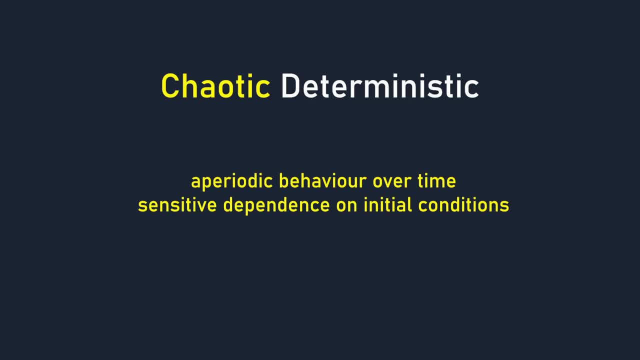 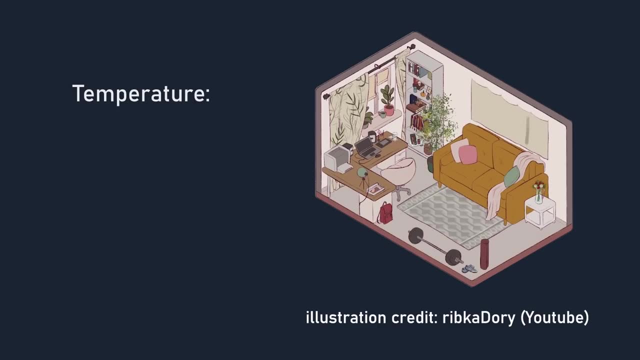 they behave and are extremely sensitive to small changes in the initial conditions. Of course, it's impossible to find out what's happening in the real world, but it's possible to predict what's happening in the future. You can find out the exact parameters of the real world with zero margin of. 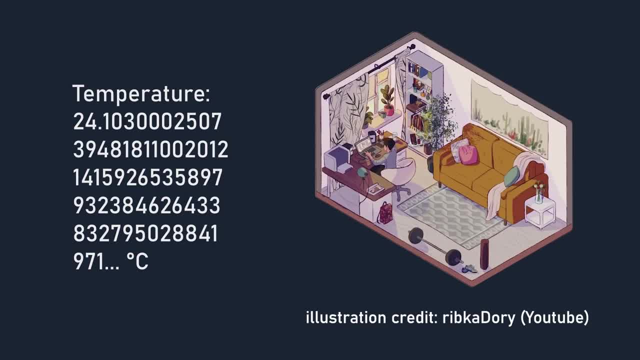 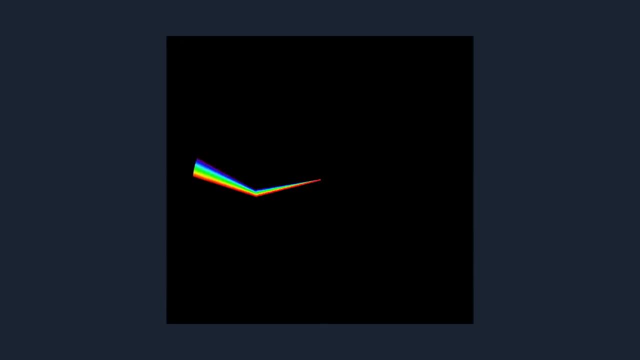 error such as knowing the temperature of a room to infinite decimal places and any small differences in the initial conditions will gradually become larger and larger differences As a result. one of the most important tasks when dealing with chaos is to find out: after what period of time is it? 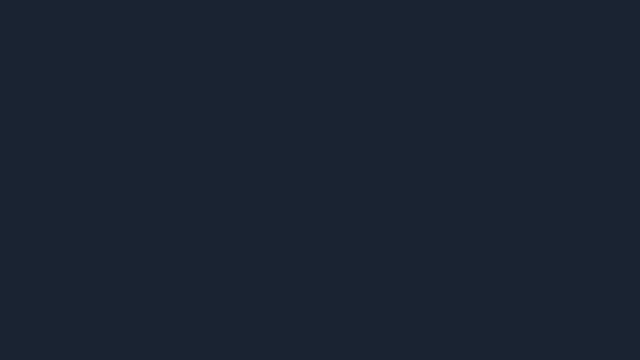 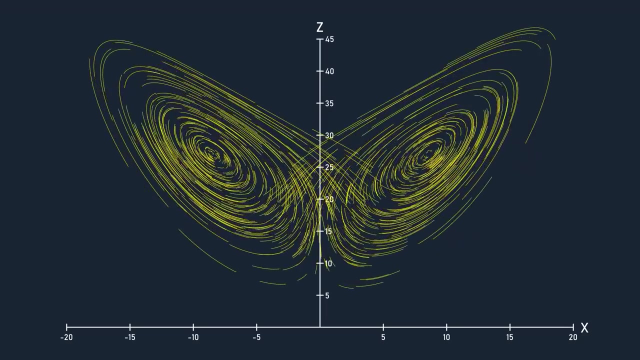 simply not worth it to predict the future. But chaos goes much deeper than simply being unpredictable. The whole phenomenon and field of study is just a matter of time, And it's not ever easy to understand the complexity of chaos. Chaos has its roots in differential equations and 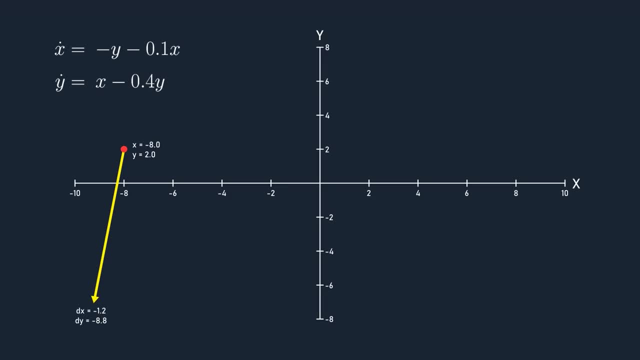 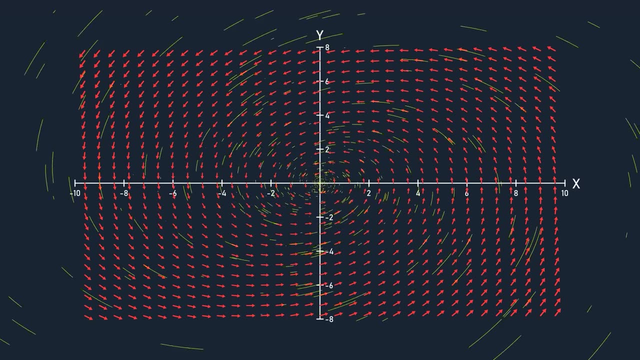 dynamical systems, the very language that is used to describe how any physical system evolves in the real world. This video aims to tell the story of chaos, step by step, from simple nonchaotic systems to different types of attractors, to fractal spaces and the language of unpredictability. 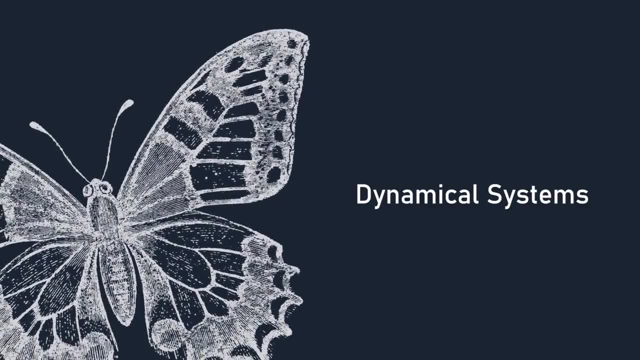 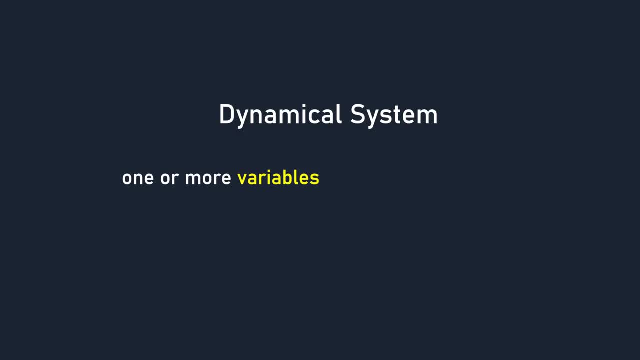 The real world has its roots in differential equations and dynamical systems. The very language involves one or more variables that change over time according to autonomous differential equations. For example, let's say there is a system that has two variables, x and y. x dot is the rate of change of x as time changes, and y dot is the rate of change of y as time. 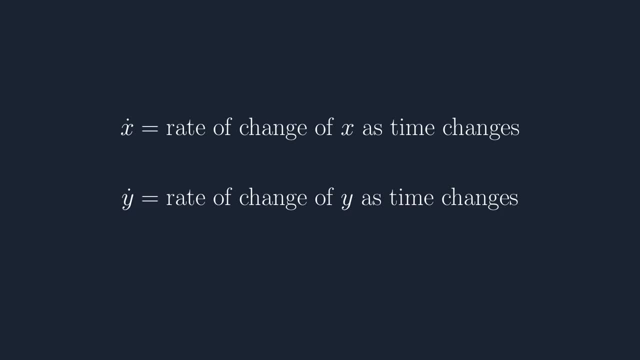 changes. Keep in mind that, even though it doesn't show it, x and y depend on the independent variable of t, which stands for time, and this dot notation is special in that it can only be used when the independent variable is time. However, notice how the differential equations that describe x dot and y dot don't actually 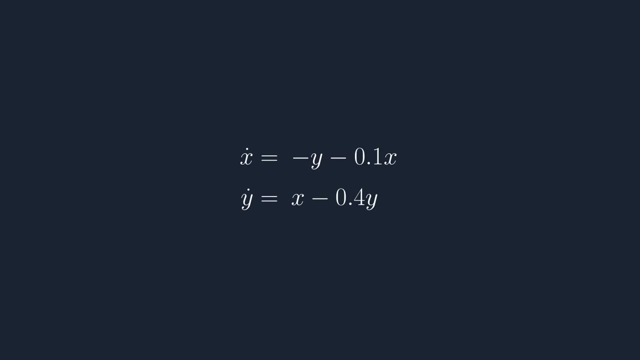 involve t and only contain x and y as variables. This makes them autonomous. Each combination of x and y only corresponds to one combination of x dot and y dot. As a result, there is a very convenient geometrical and visual way of representing a dynamical 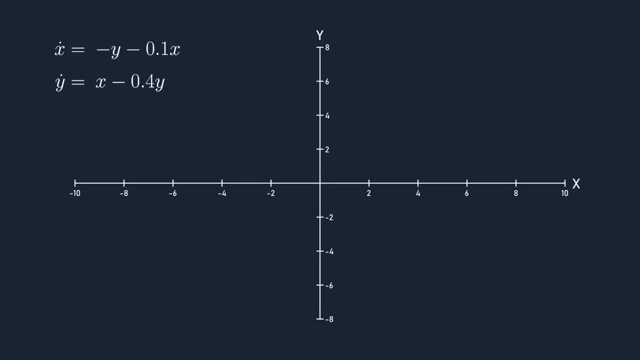 system known as the phase space. This is a cartesian space where the axes are the system's variables. Each point in the space is a unique state of the system and has its own rate of change, which can be shown as a vector For this specific system. shown, the vector field looks like this: Let's scatter a bunch. 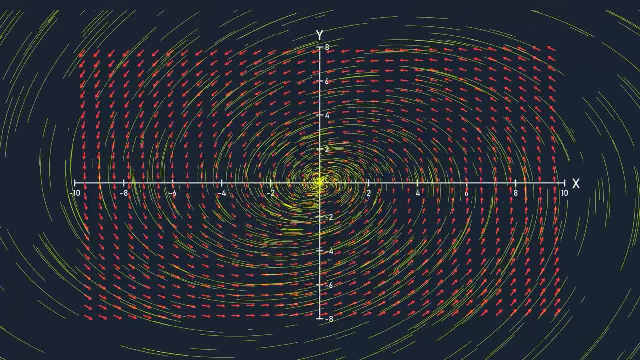 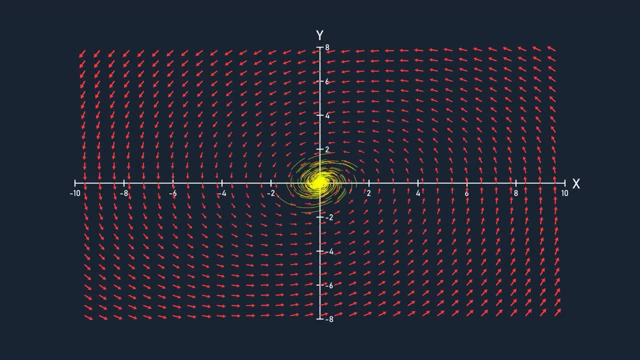 of random points around to represent different possible states and see how they evolve and move around. Seems like they all spiral towards the center, But overall it's definitely high on here, which makes it'd be lame if Words obvious that the vector field suddenly turned upside. 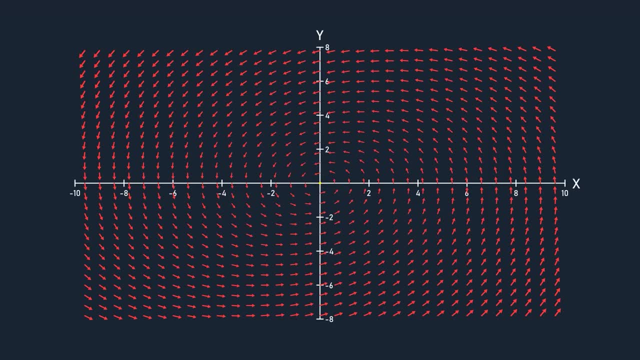 down with the underlying matrix location. Finally, from the top of the topic, the vector field looked like this. Now let's try to draw the currentMeicos. This brings us to our next topic. an attractor is a set of points: Hindi and k-R än Medal. 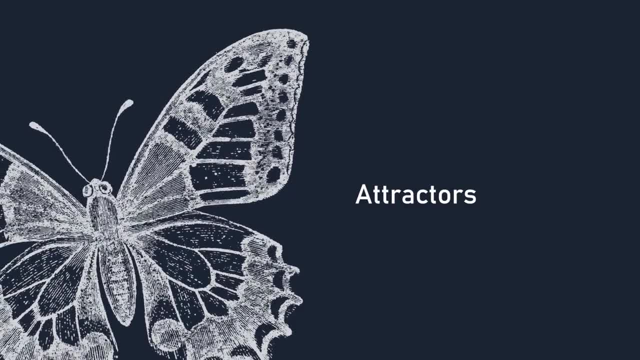 and theissions that connect with downwards as they swivel between the vertical axis. An attractor is a set of points in the center in which a constant positive force is a constant positive range in a stack value. By starting at the right one method of 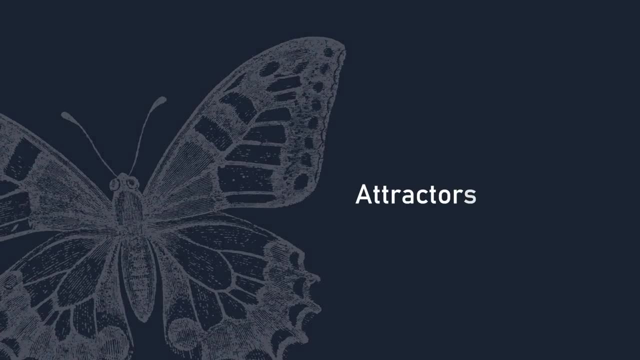 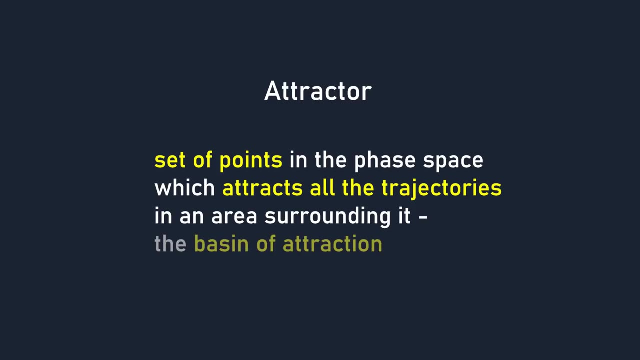 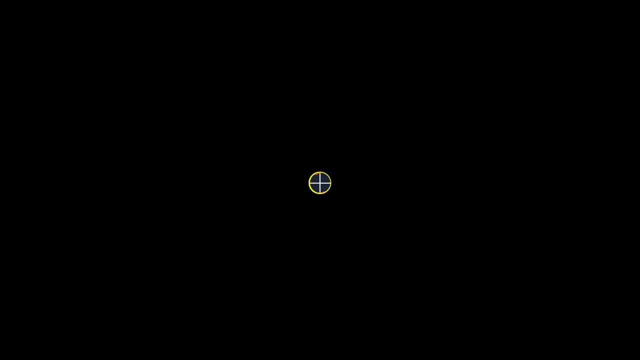 An attractor is a set of points in the phase space which attracts all the trajectories in a certain area surrounding it, known as the basin of attraction. Here the attractor is just the origin and the basin of attraction is every point in the space. 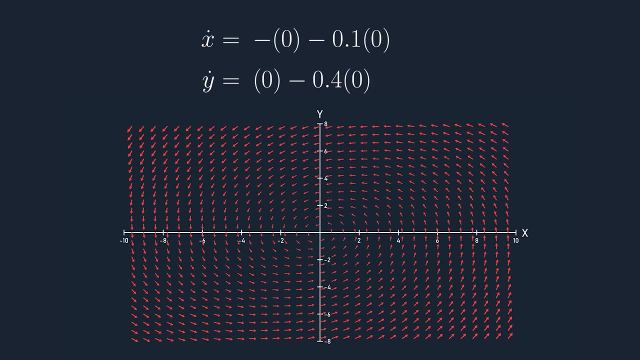 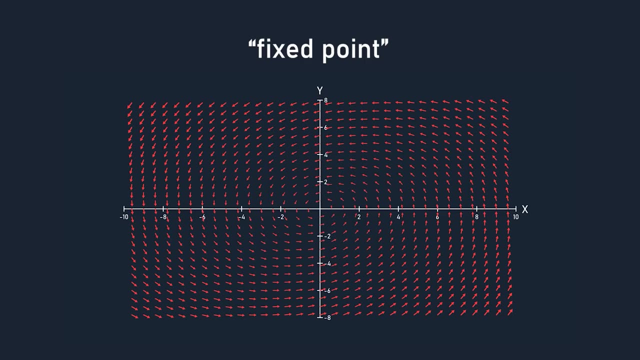 Notice that at the origin, where x equals 0 and y equals 0, x dot and y dot equals 0 too, That makes it a fixed point, because any point there will stay there forever due to it having a rate of change of 0.. 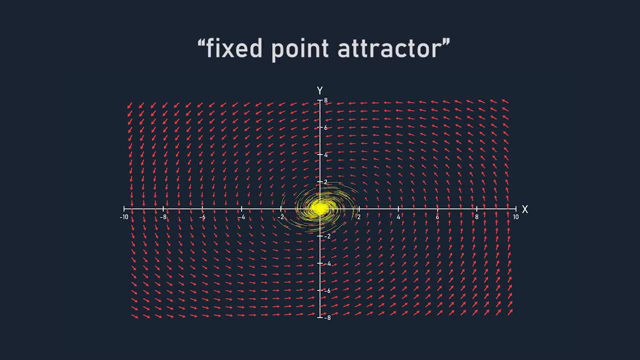 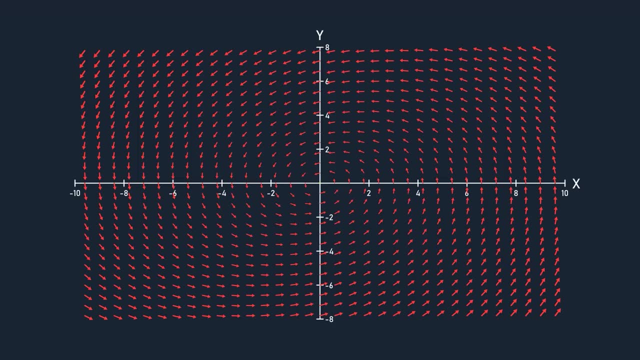 Since it's also an attractor. it's a fixed point attractor. Trajectories that get sucked into any attractor never get to escape. This seems to reflect some sort of inevitability and predictability that the system will always end up a certain way, no matter what. 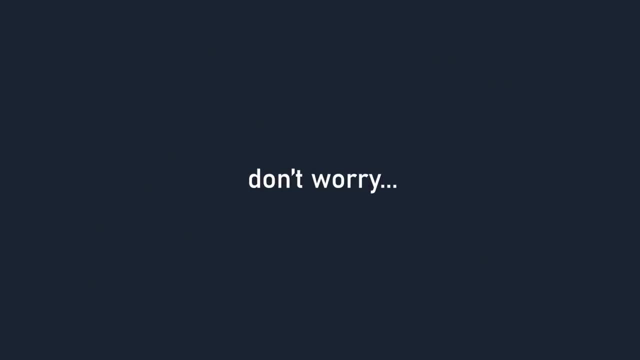 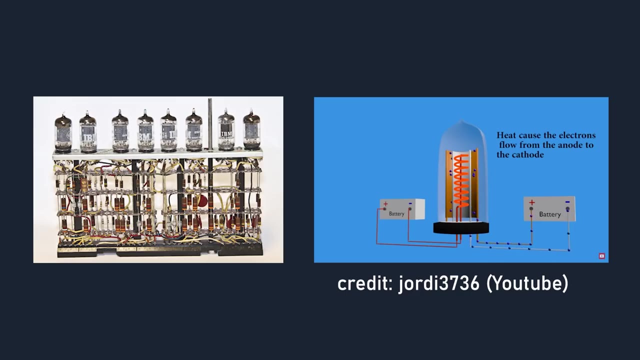 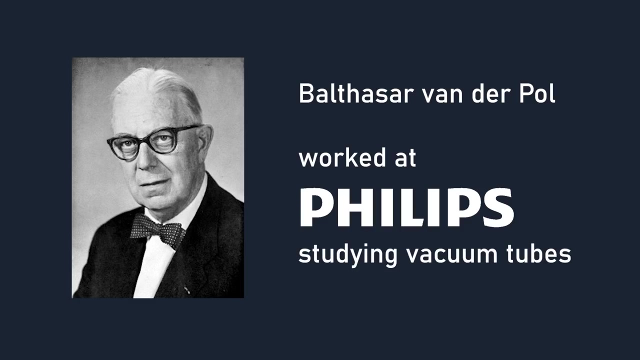 How could this be related to chaos? Well, don't worry, there's also other types of attractors. There was a time when computers were made using vacuum tubes. Balthazar van der Pole worked as an electrical engineer at Phillips during the 1920s. 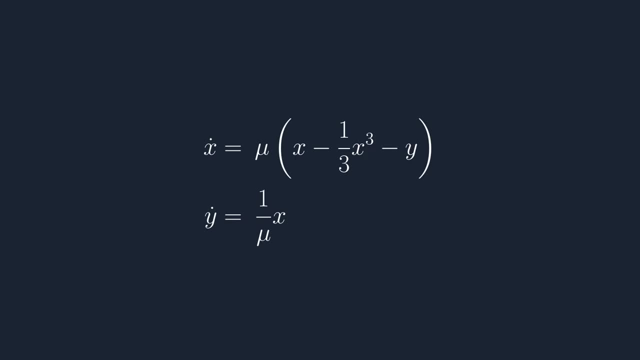 It was while studying vacuum tubes that he stumbled upon a system of differential equations that exhibited some interesting behavior and would later be known as the van der pole oscillator. The original equations had a parameter that x dot was multiplied with and y dot was divided by. 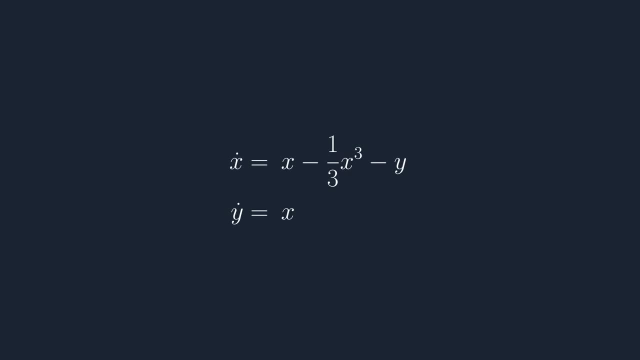 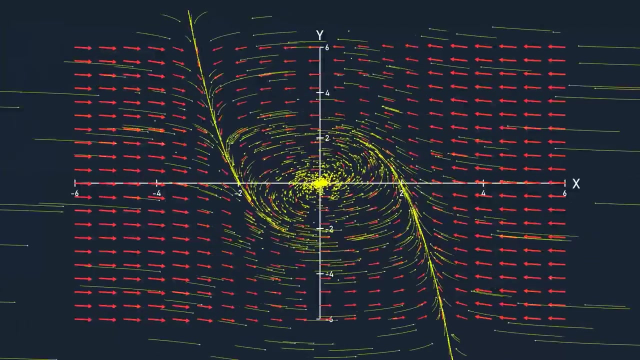 But here the parameter has been chosen to be 1.. This is exactly what happened. one for a simpler set of equations. If we plot this system's phase plane, we can see that, interestingly, trajectories everywhere seem to approach this loop around the origin. 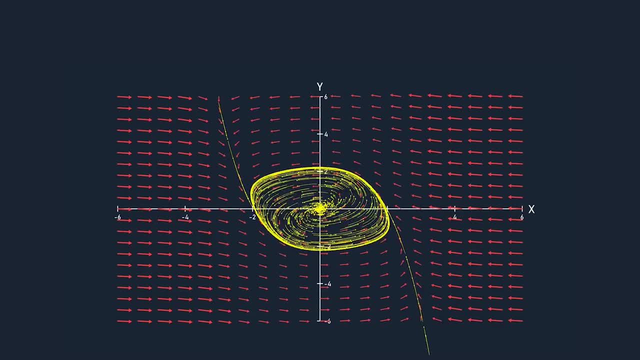 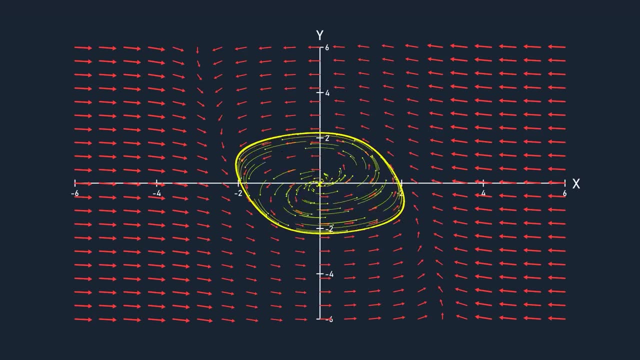 This loop is known as a limit cycle attractor and is an important example that shows us that the attraction of trajectories does not necessarily have to result in the trajectory stopping at a singular point. Limit cycles are often characterized by physical phenomena that involve some sort of oscillation. 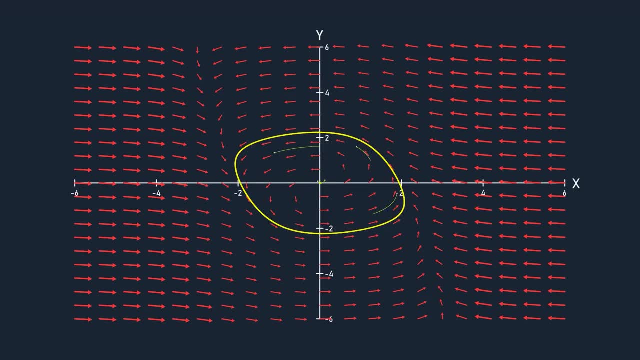 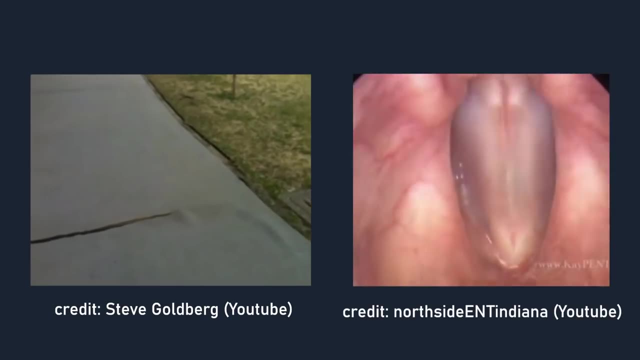 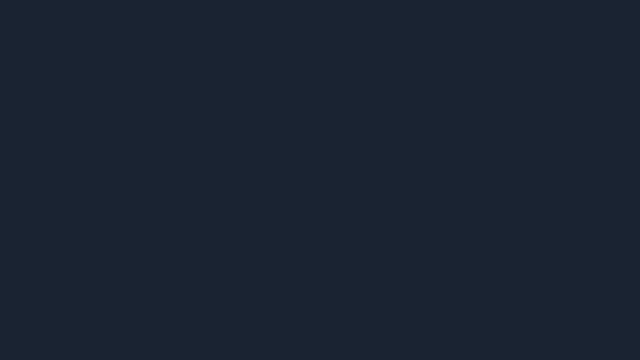 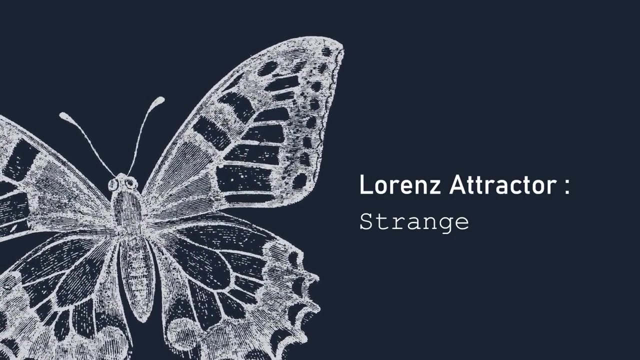 and van der Pol's equations are no different Other than electrical circuits. they have been used to model things like two tectonic plates at a geological fault or the mechanics of human vocal cords. But this is still not quite chaotic. There is two more ingredients. 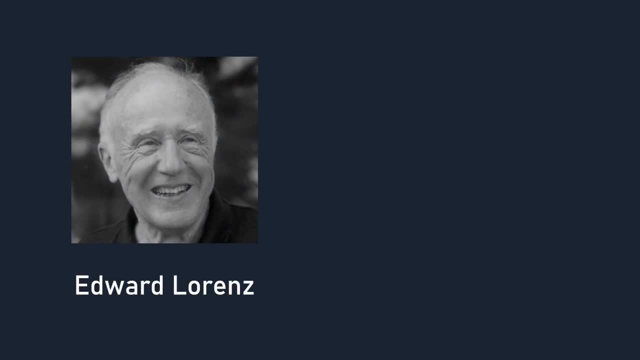 In 1963, meteorologist Edward Lorenz was developing a system called the Van der Pol's equation. In 1963, meteorologist Edward Lorenz was developing a system called the Van der Pol's equation. He developed a simulation for atmospheric conditions which involved 12 changing variables. 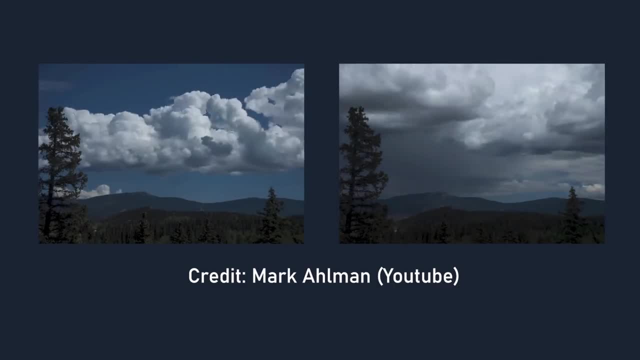 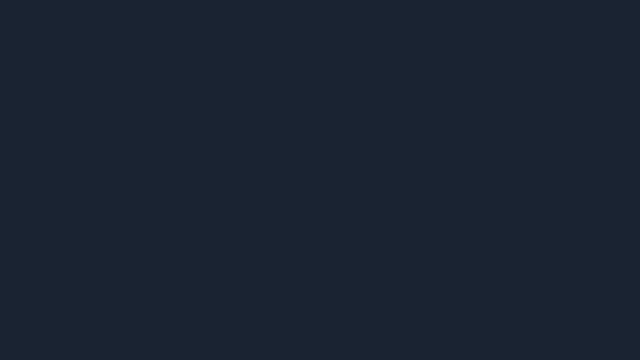 and found that tiny differences in the initial values resulted in disproportionately big differences in the state of the variables. just a short time after, Curious about this, Lorenz spent some time simplifying his simulation to only have three variables but still display this sensitive dependence on initial conditions. 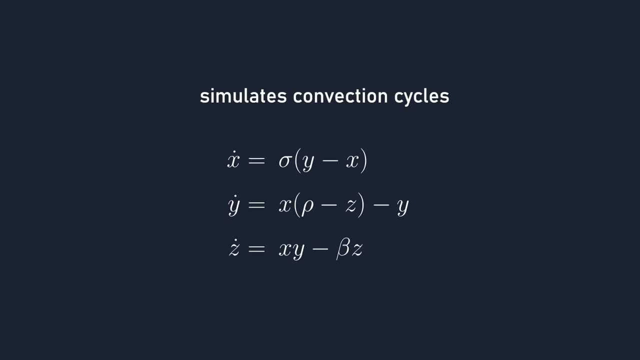 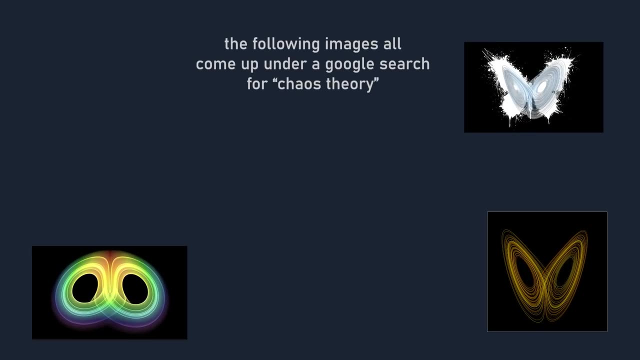 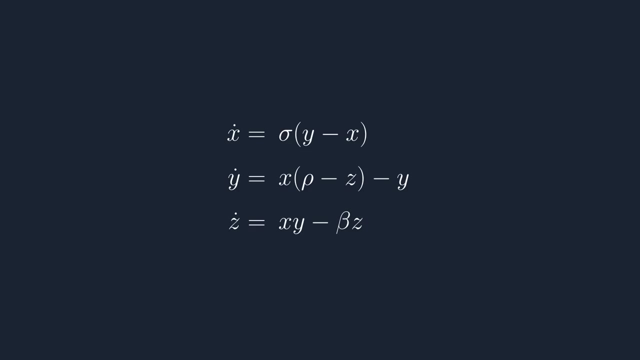 The simplified model describes convection cycles in the atmosphere and is now known as the Lorenz system. It's the poster child of chaos theory and is sometimes almost synonymous with the butterfly effect or the field of chaos theory itself. It even looks like a butterfly. 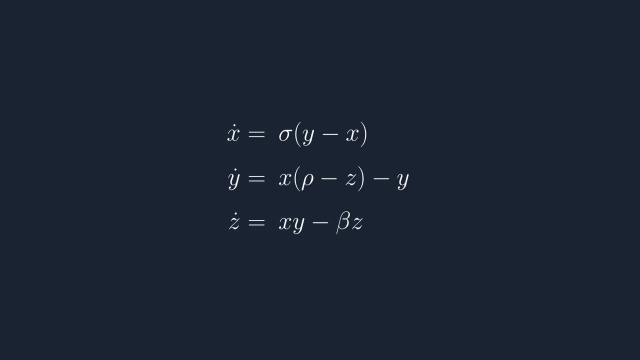 The Lorenz equations have a few parameters that can be tweaked to alter the behavior of the system, but we'll be using values of 28,, 10, and 8 over 3.. This is what's known as a strange attractor, and here's what that means. 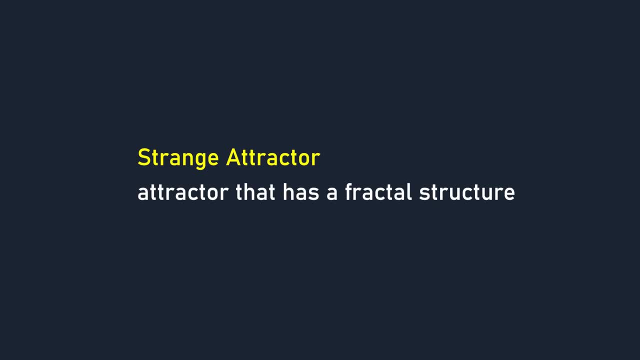 A strange attractor is one that has a fractal structure. No point in the space between a fractal structure and a fractal structure, No point in the space is ever visited more than once by the same trajectory. If that happens, the trajectory would travel in a predictable loop and no two trajectories. 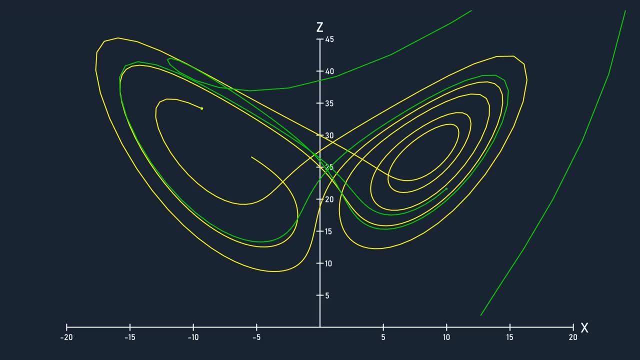 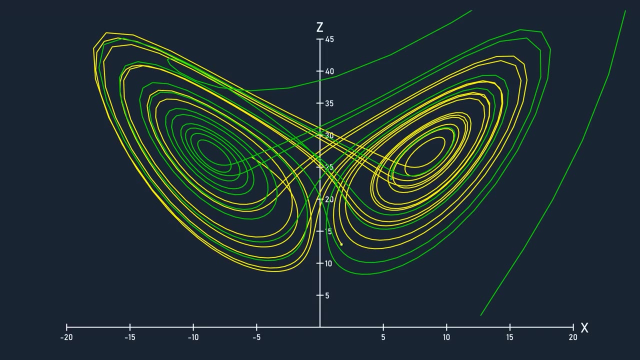 will ever intersect. If that happens, they would merge into the same path, giving two different sets of initial conditions the same outcome. Think about what that means. A single trajectory will visit an infinite number of points in this limited space, and this limited space will have an infinite number of trajectories. 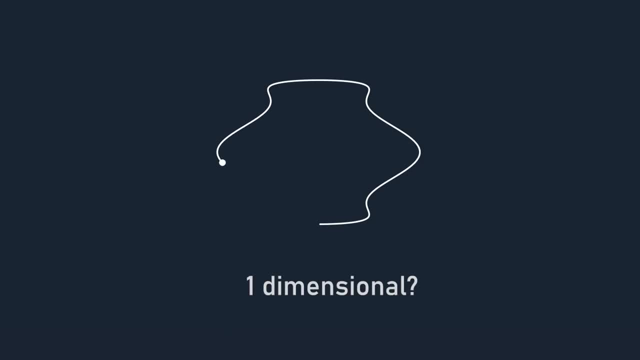 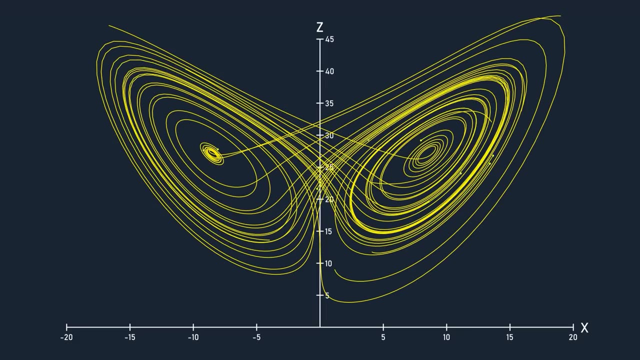 Now, trajectories are just curves, so they should be one-dimensional, right. But how come, no matter how much you zoom in on this attractor, you can always find more and more trajectories everywhere? That's why this attractor is said to have a non-integer dimension. 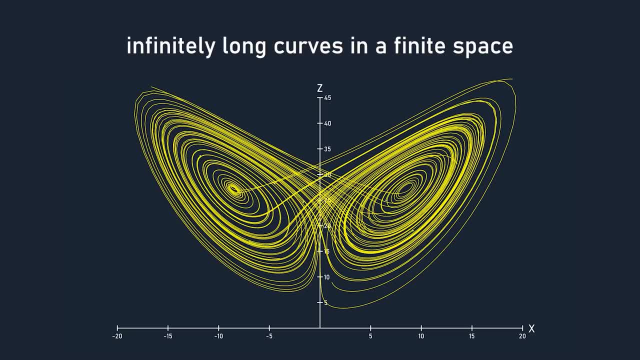 It's made up of infinitely long curves in a finite space which are so detailed that they start to partially fill up higher dimensions. It's not one-dimensional, two-dimensional or three-dimensional, It's just one-dimensional. Its dimension is somewhere in between. 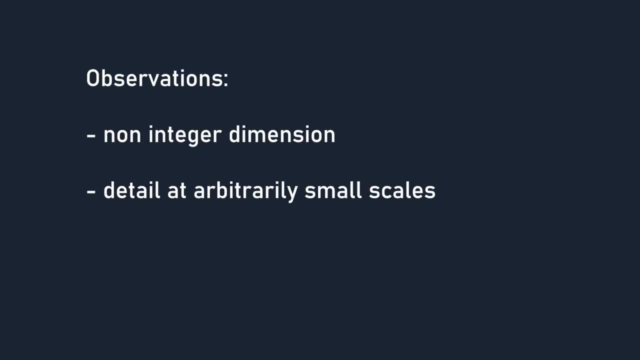 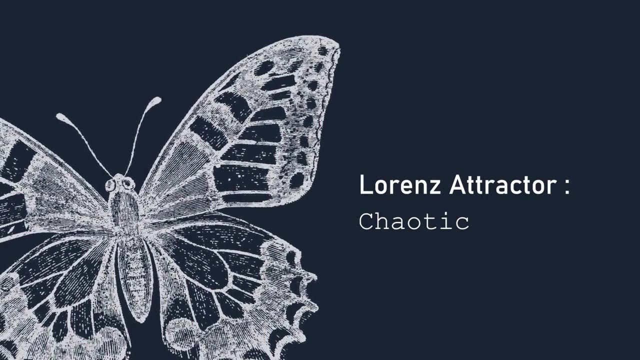 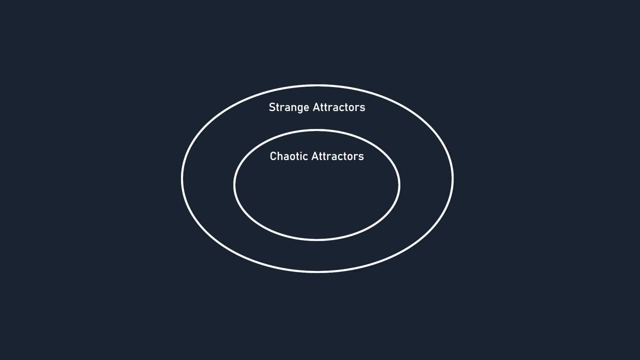 As a result of this non-integer dimension and detail at arbitrarily small scales, the set of points in the Lorenz attractor is a fractal space, And that's why it's a strange attractor. A strange attractor isn't necessarily chaotic, but a chaotic attractor will always be strange. 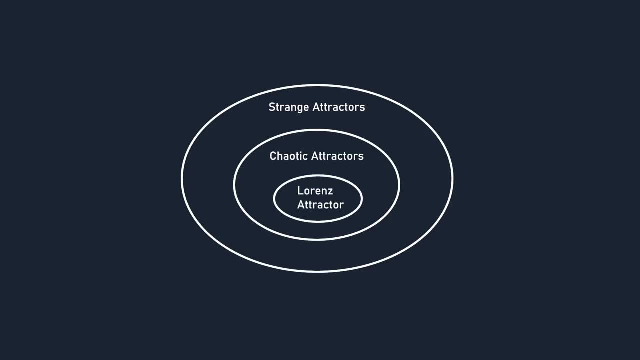 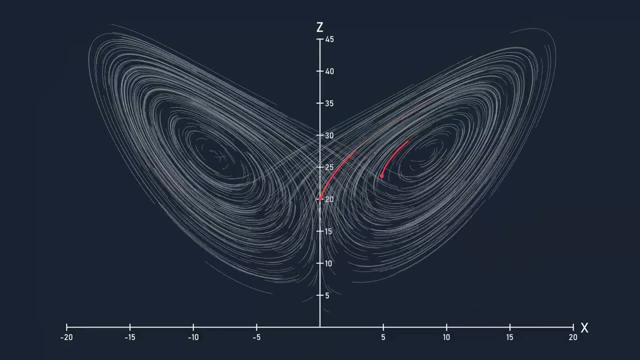 And the Lorenz attractor is a strange chaotic attractor. Watch what happens when I highlight two trajectories that are initially a very small distance apart. It doesn't take long for them to diverge so much as to be on completely different paths. 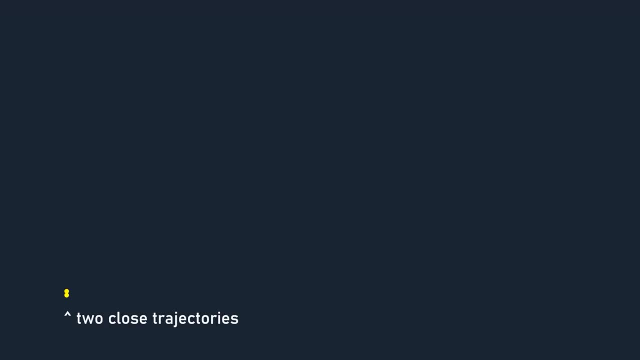 It turns out that in the early stages of this divergence, when the two trajectories are close to each other, the distance between them increases exponentially. After a time of t, the resulting difference is the initial difference times e to the power of lambda t. 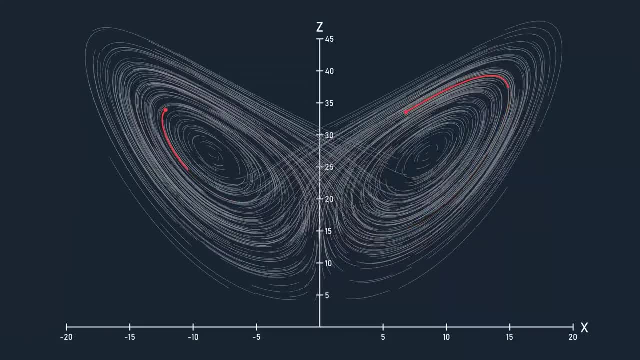 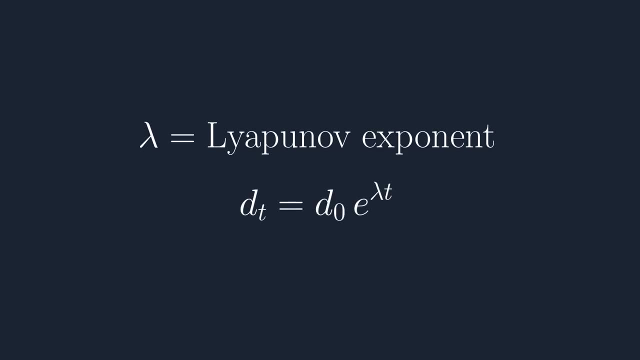 Up until a certain point, of course, since the attractor is only so big. Here, lambda stands for an important value known as the Lyapunov exponent, Since it's the factor of the exponent of e. if it's positive, then any distance between 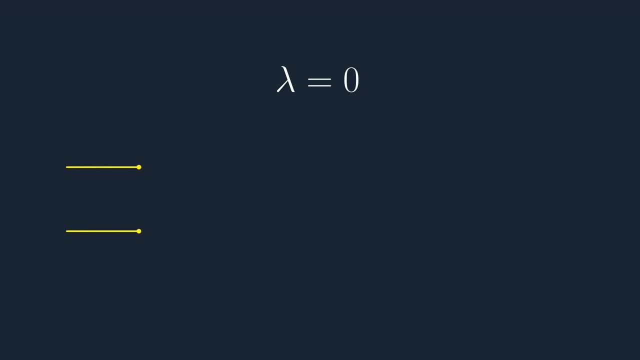 trajectories will increase exponentially. If it's equal to zero, then the distance will stay constant, And if it's negative, then the distance will converge to zero. There isn't a way to find the Lyapunov exponent by just looking at the expression. 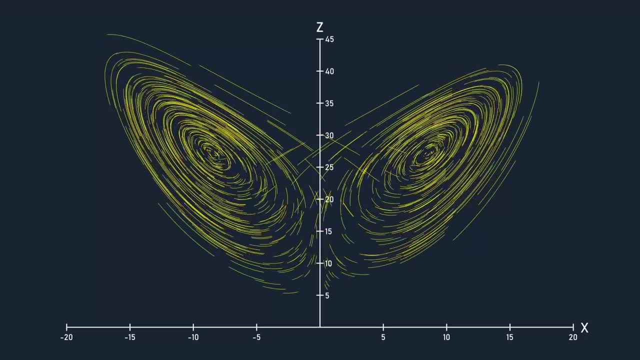 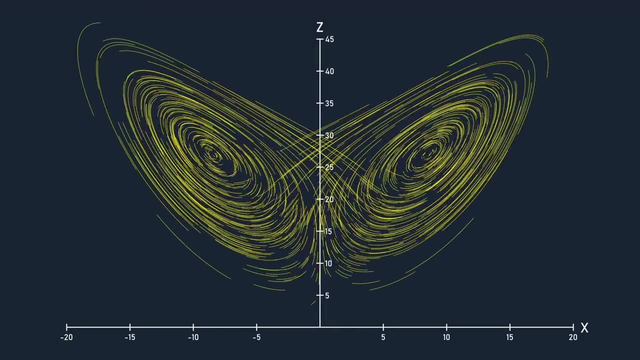 Instead, we can use the language to find out what it's actually equal to. Let's see equations. It is measured by actually running the simulation, keeping track of many pairs of trajectories and finding the average rate of change in their distance, But it provides. 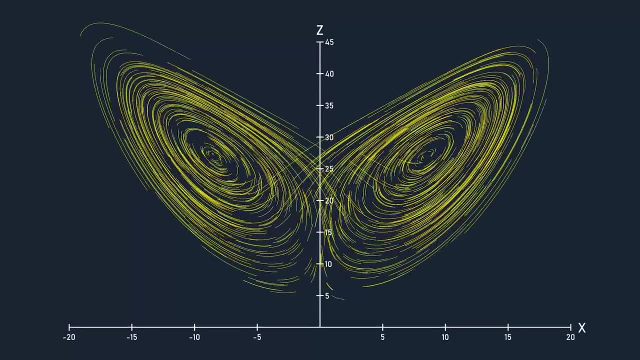 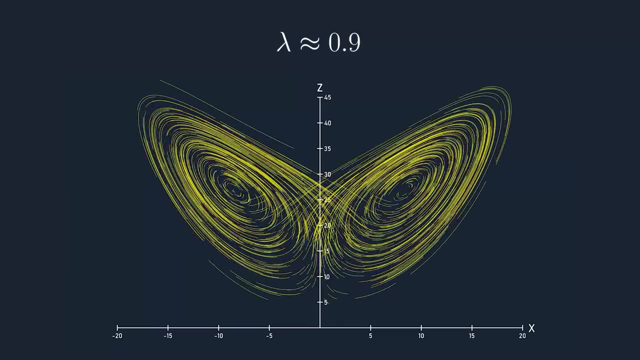 a simple metric to communicate how chaotic a system is. As long as the Lyapunov exponent is larger than zero, the attractor will be chaotic and it's equal to about 0.9 for the Lorenz attractor. That's how we can figure out the duration of time in which predictions 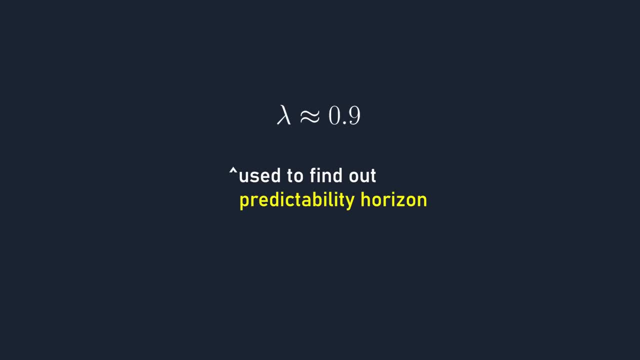 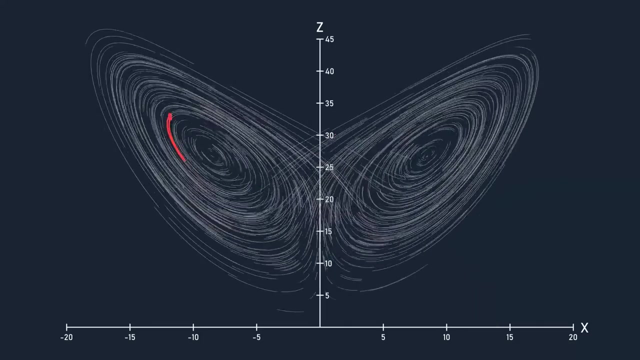 are valid, otherwise known as the predictability horizon. Rearranging the previous equation, we can see that this is how it can be found: given the initial error, delta 0, and a maximum error that we are willing to allow, a In the Lorenz system after a time of just 10,. 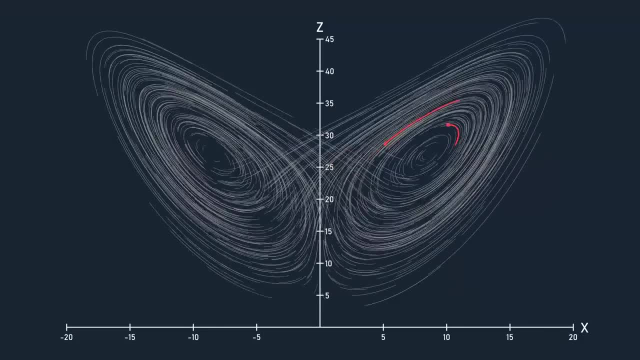 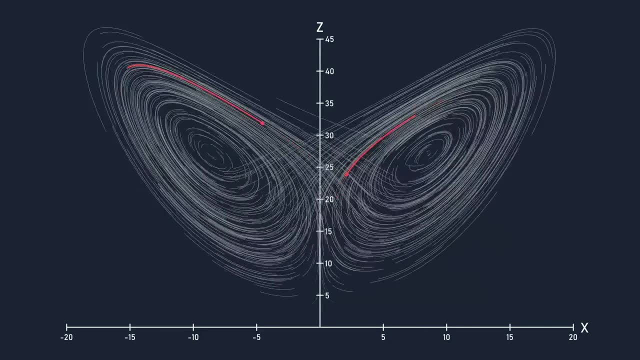 any error would have multiplied by more than 8000.. To get an idea of how hard it is to make accurate predictions over long periods of time with this exponential divergence, we need to calculate the duration of time. In this case, we need to calculate the duration. 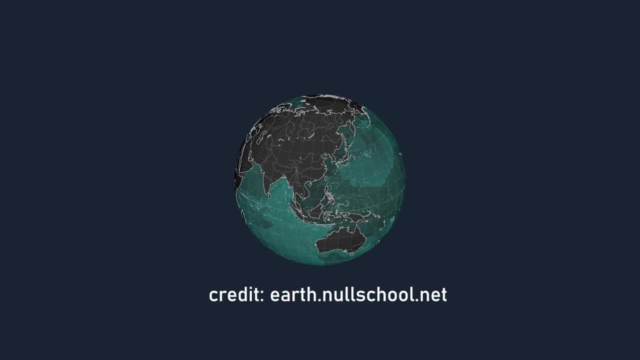 of time. In this case, we need to calculate the duration of time. In this case, we need to calculate the duration of time. Let's say you had a simulation that predicts where ocean currents flow and you wanted to keep the error less than 1000 meters If you ran. 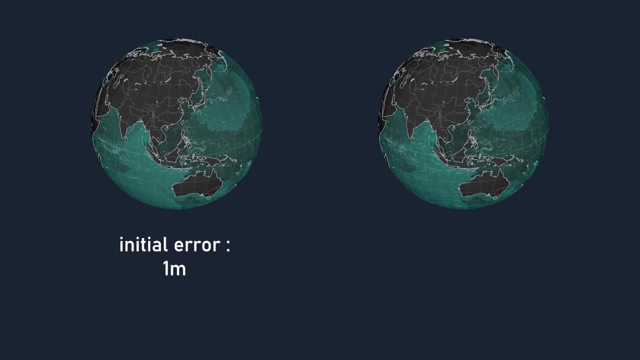 it twice: once with an initial error of 1 meter and once with an initial error that was a million times smaller, at 1 micrometer. how much longer do you think the simulation with the smaller error would stay below the margin of error? Well, let's write the expressions.